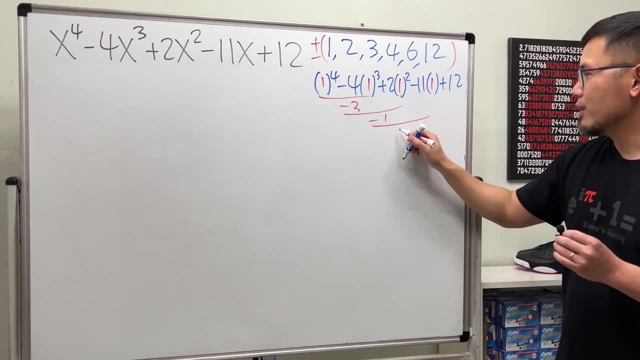 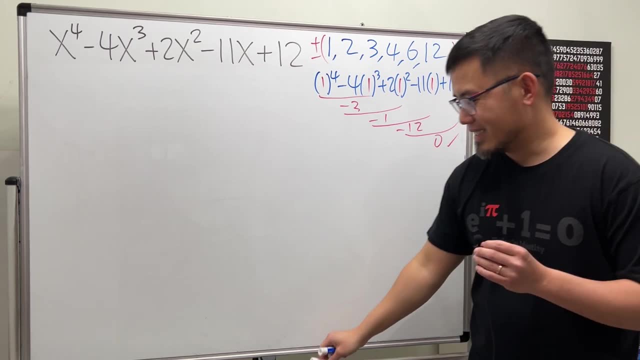 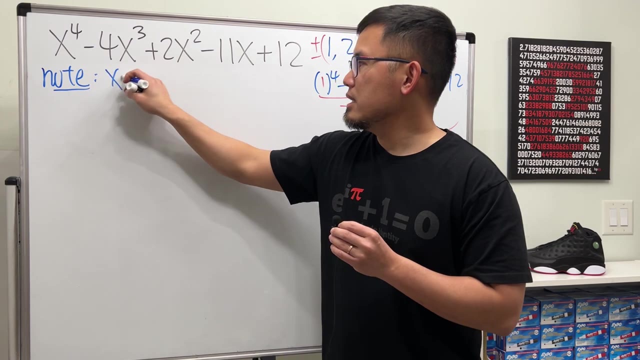 and then plus 2 is negative 1, and then minus 11 is minus 12, and then, lastly, you add the 12.. So it's indeed equal to zero. That means we can be happy and come back here and say: note that x equals 1, is a zero of this polynomial and 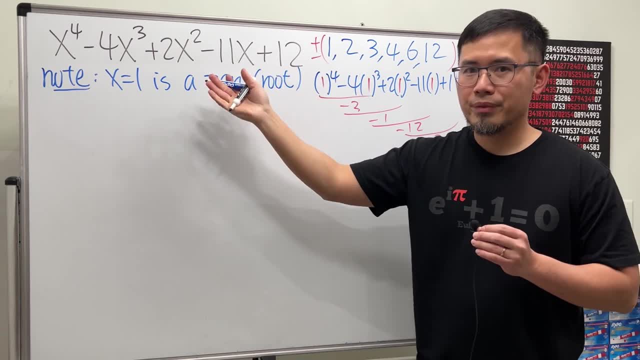 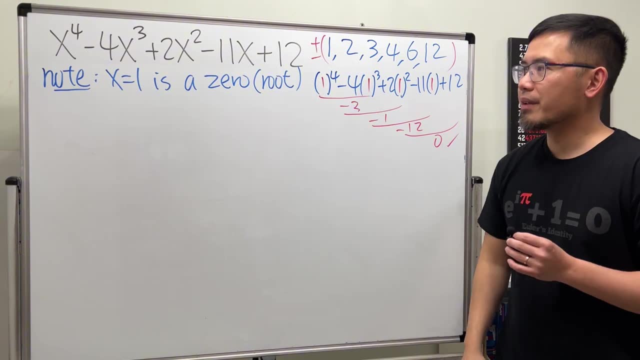 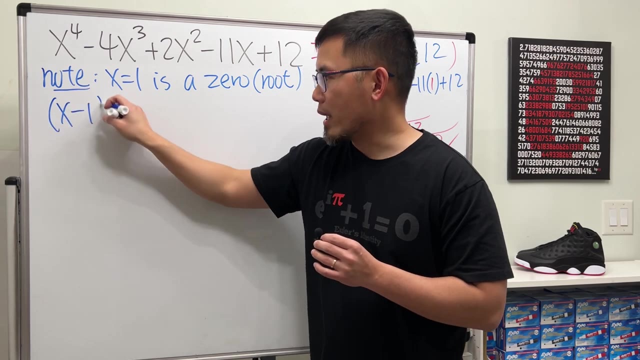 sometimes people also call this a root of the polynomial. It just means that when you plug in this number into all the axes, at the end result we get zero. Furthermore, we know, once we have this, we can say this polynomial has a factor x minus 1.. 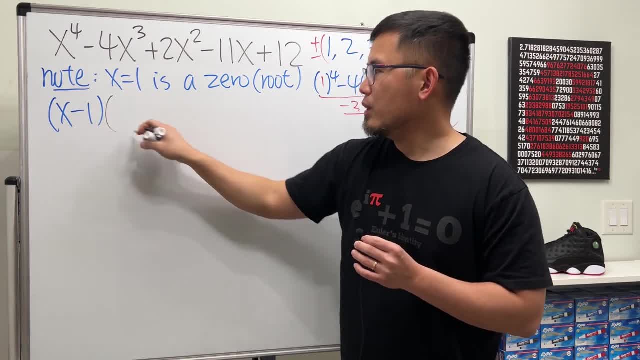 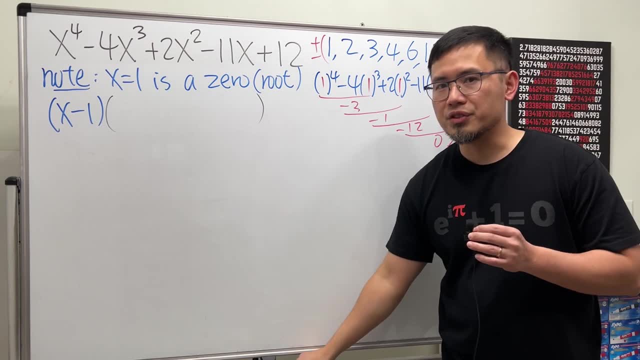 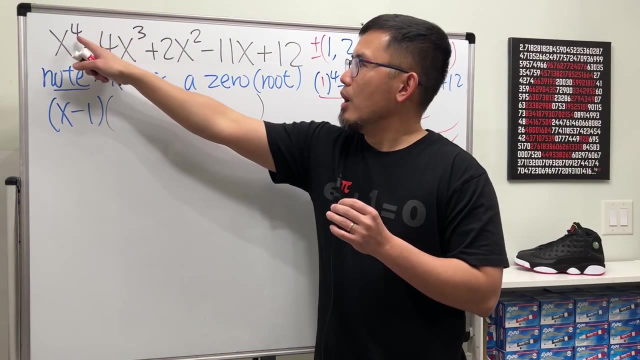 Now you just move the 1 to the other side and we'll just have to find out the other part And to do so, this is where we have to use the sensitivity feature, And to do so I'm just going to draw like a half box like this: First notice: all the powers are present: 4, 3, 2, 1 and then no x. 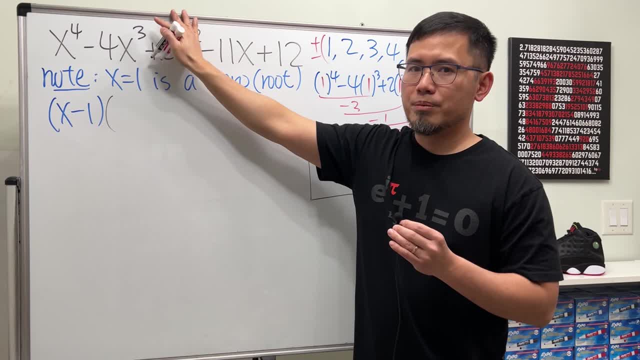 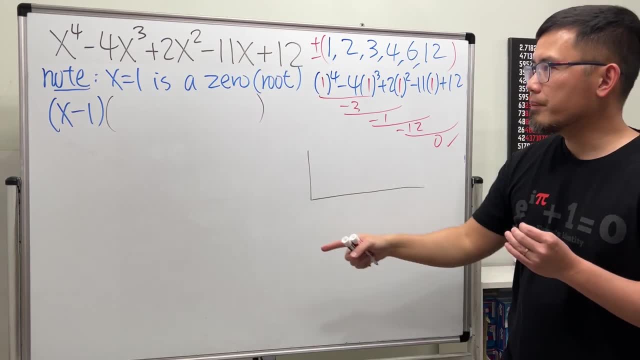 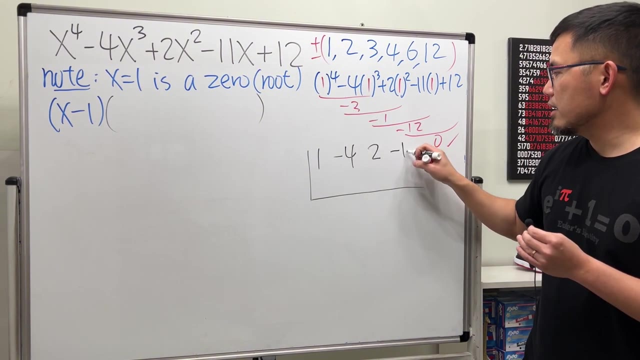 Sometimes you may be missing a like x squared term. In that case you have to use zero x squared. But we don't have to worry about that. Let's just go ahead and write down the coefficients right here We have 1, and then negative 4,, 2, and then negative 11, and the last one 12.. 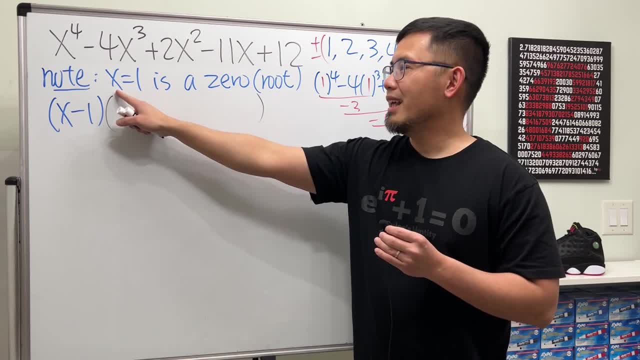 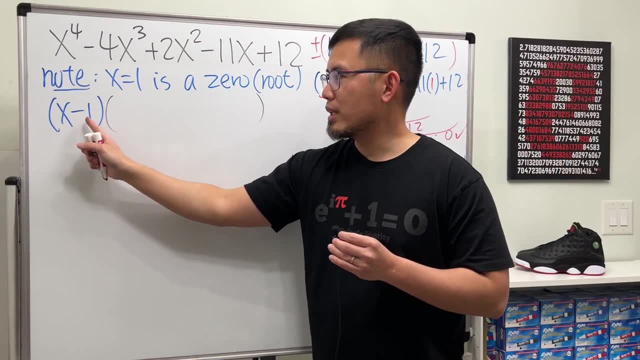 Then we are going to see that right here: x equals 1 is a zero. Go ahead and put that 1 right here. Sometimes, if you are looking at this, just make sure that you do the opposite of negative 1.. 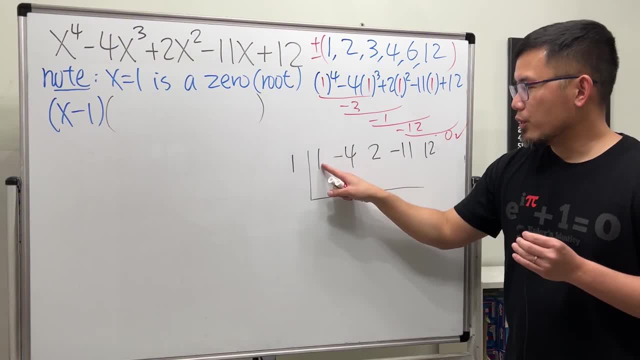 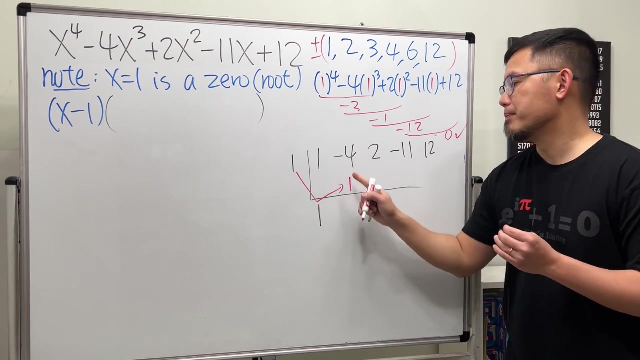 And here we go. First you bring down the 1 right here, and then we are going to just do this: 1 times this 1, and then put it here. alright, 1 times 1 is 1.. You put it here, and then we are going to add them up. 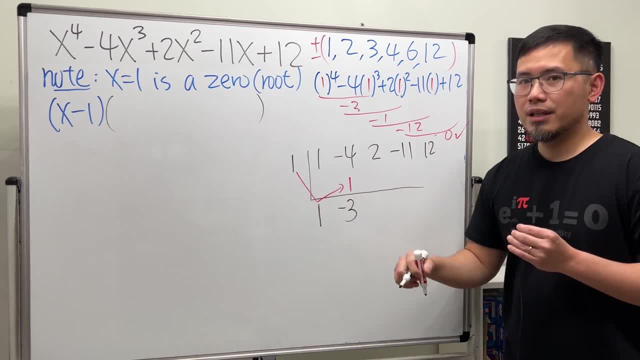 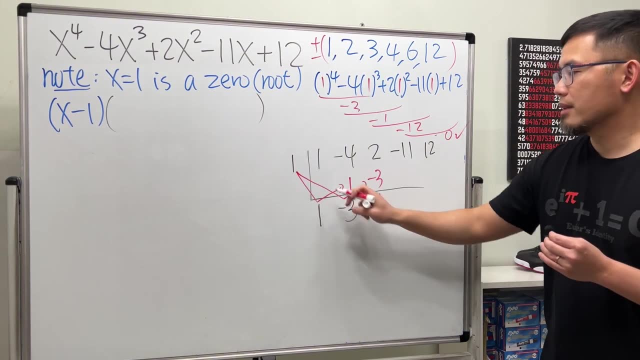 Negative: 4 plus 1 is negative 3.. And then continue: 1 times negative: 3 is negative 3.. And then you add this and that which is negative 1.. Continue 1 times negative. 1 is negative 1.. 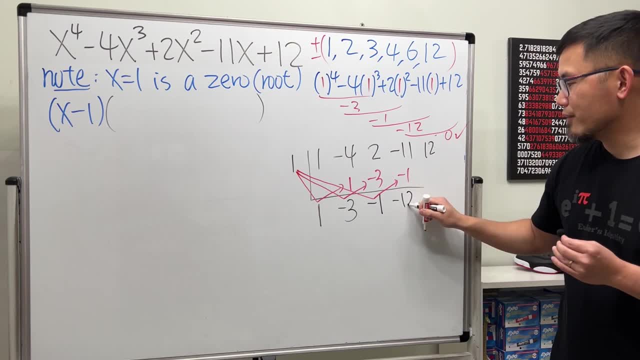 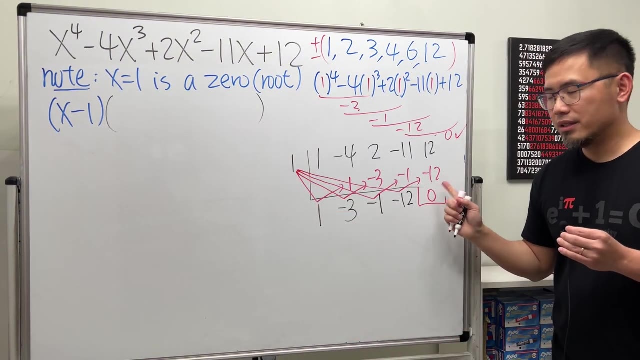 And then this and that is negative 12.. Lastly, 1 times negative 12 is negative 12.. When we add them up, we get zero. If we have a zero, the final result here must be zero. This is the remainder, and then this right here will tell us the factor. 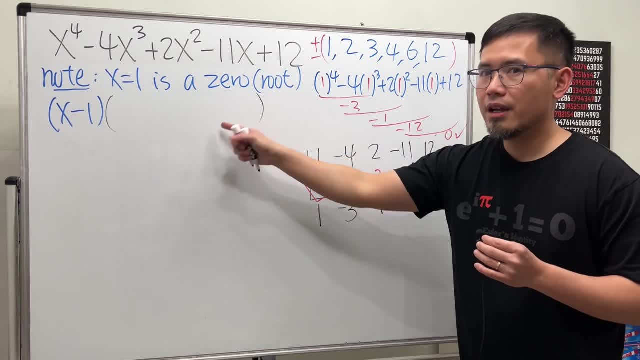 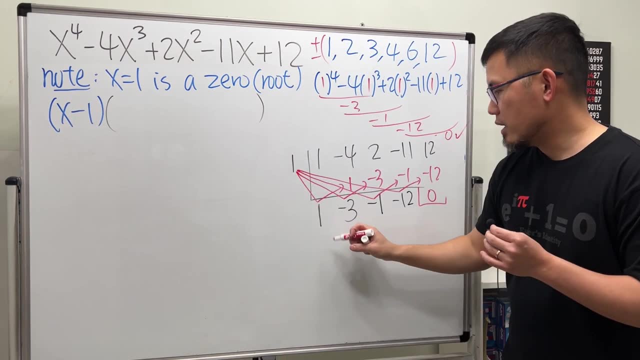 These are the coefficients of our factor, and remember the power will go down by 1. Because we factored it out, x to the first power, So this right here will be 1x to the third power And then minus 3x squared. 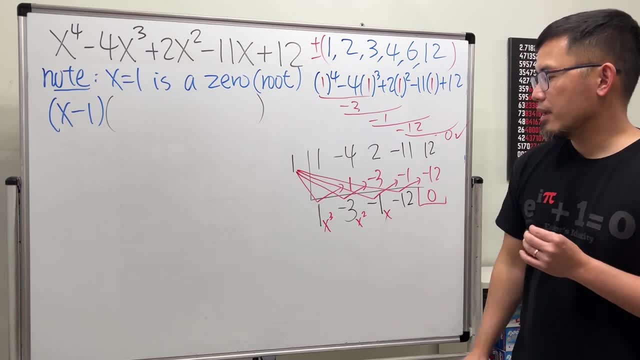 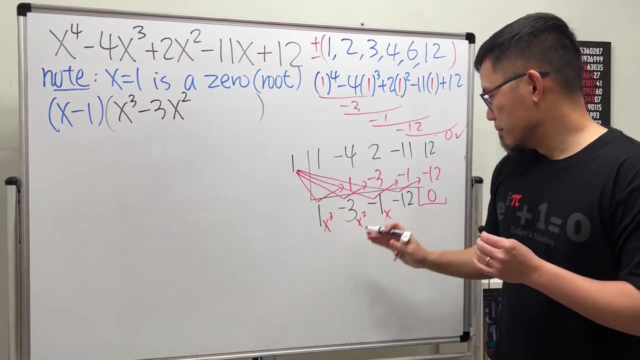 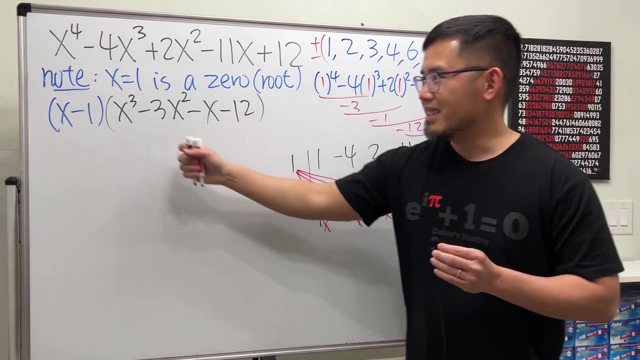 And then minus 1x, And then the constant term. So let's put that down: x to the third power, minus 3x, squared Plus minus 1.. And then minus 12.. Cool, Now what? Yep, now we have to focus on how we can factor a full-term polynomial. 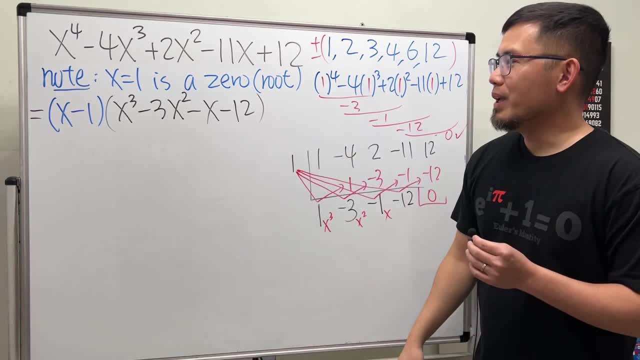 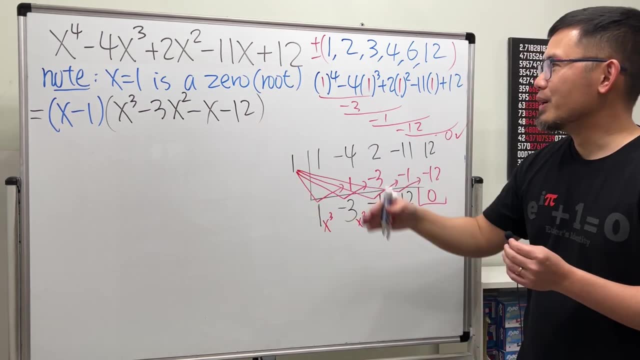 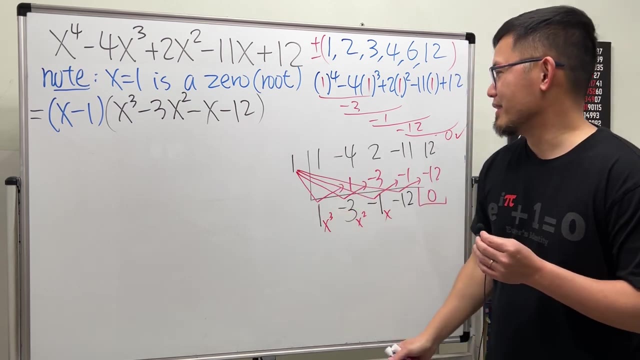 To do so, we are just going to use the rational 0, 0 again And, yeah, we have negative 12.. So you can try again. I will just tell you guys that 4 is a root for this right here. 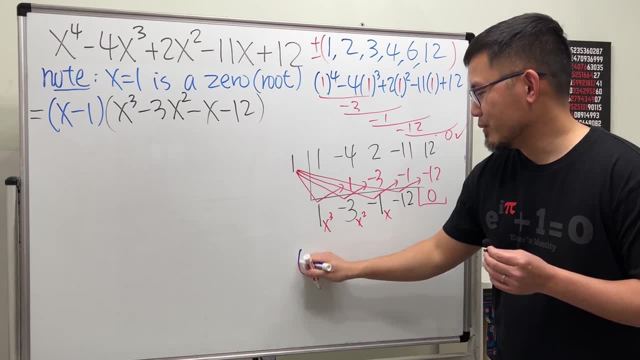 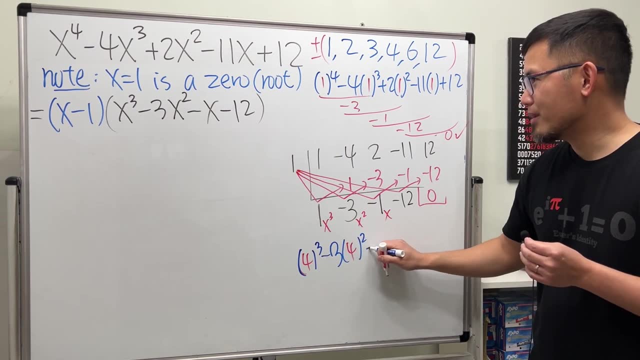 So I'm just going to show you guys real quick. So if we do 4 to the third power minus 3, times 4 to the second power minus 4.. And then minus 12.. Let's see This right: here is 64.. 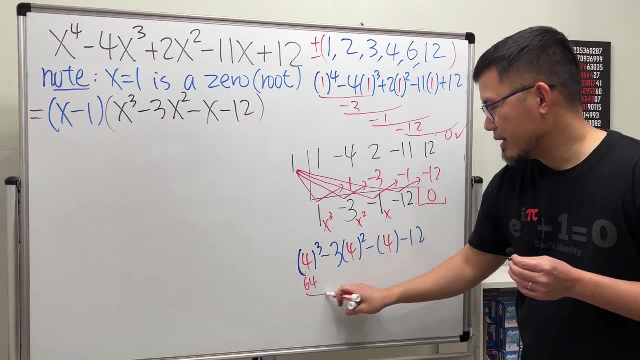 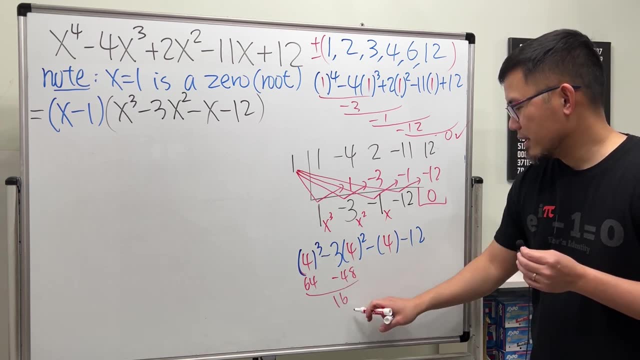 And then this is 16. That's minus 48.. So together that's positive 16. And then minus 4 is 12. And then minus 12 is 0. So 4 does work Sometimes. of course, you will have to just keep trying for a few times. 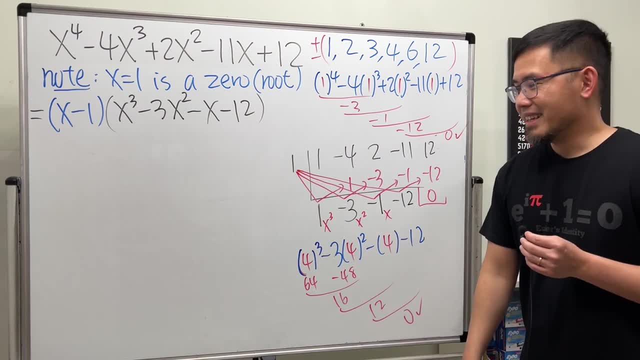 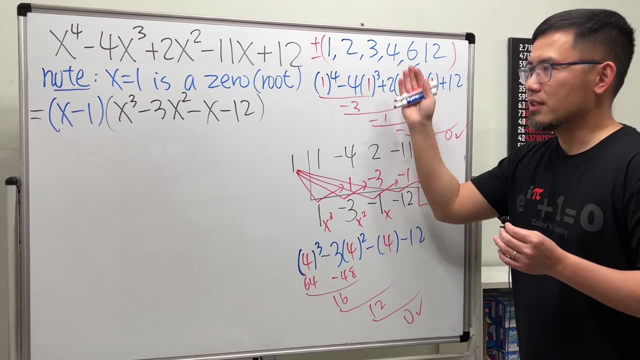 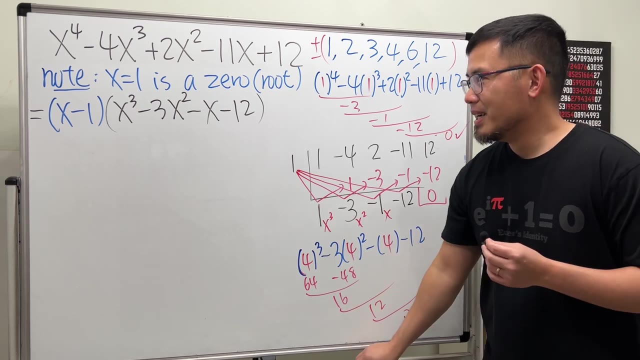 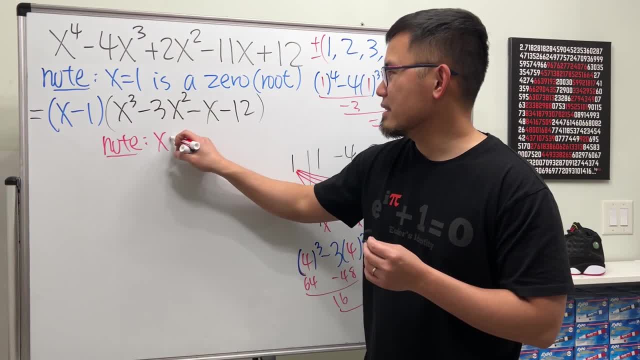 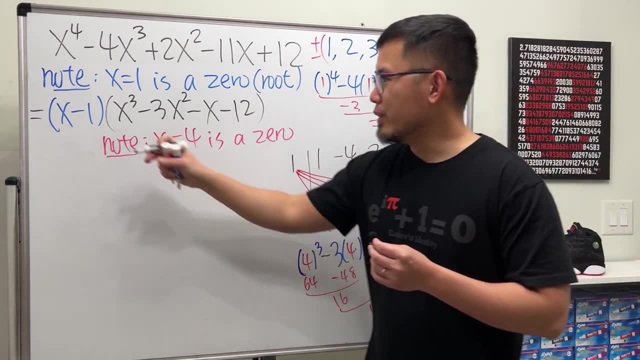 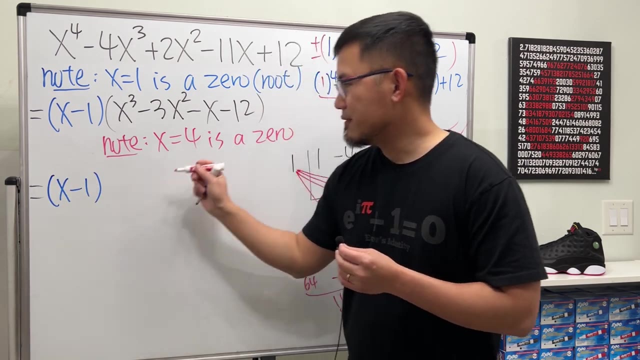 note this time: x equals 4 is a 0 for this right here. So that means we know this right here is equal to our first factor is still x minus 1.. And the next factor will be minus 4.. And we just have to figure out. 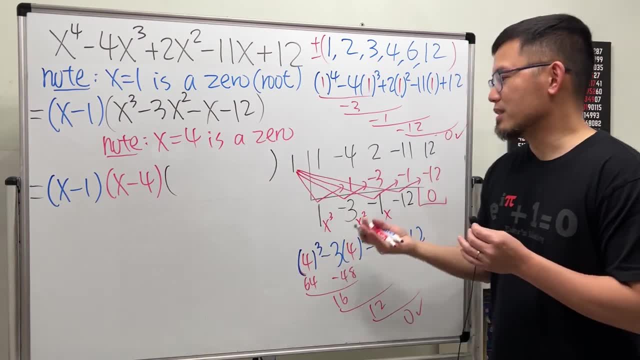 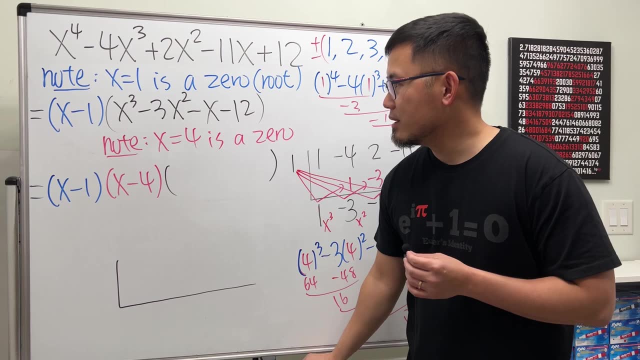 what do we have left? And to do so again, we will do the sensitivity efficient. So let me just put it down right here real quick for you guys. I'm just going to write down the coefficients, And all the powers are present. 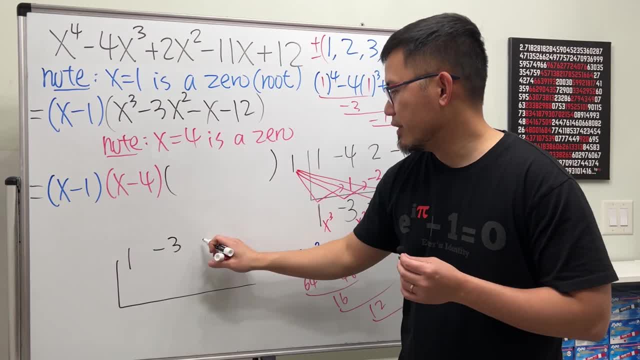 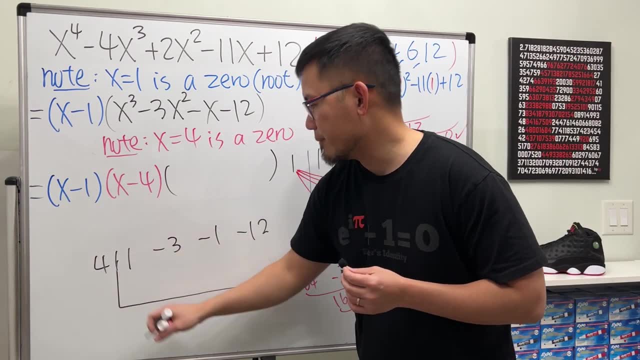 So we can just write down 1, negative 3, negative 1, and negative 12.. This time we are using 4.. So put a 4 right here And here we go, Bring this down, And then we do 4 times 1,, which is 4.. 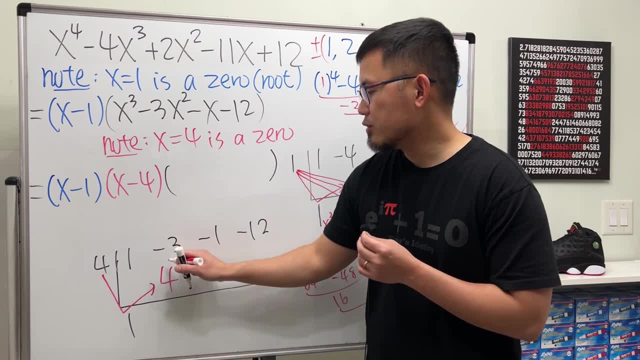 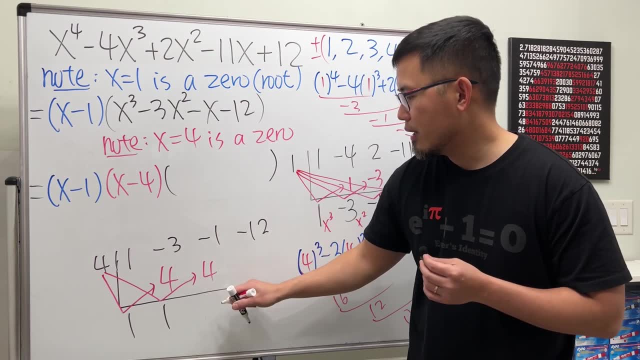 Put it here, And then we add them: Negative 3 plus 4 is positive 1. And then continue This times: this is 4.. Put it here: is 4.. And then we get 3.. Continue This times: this is 12.. 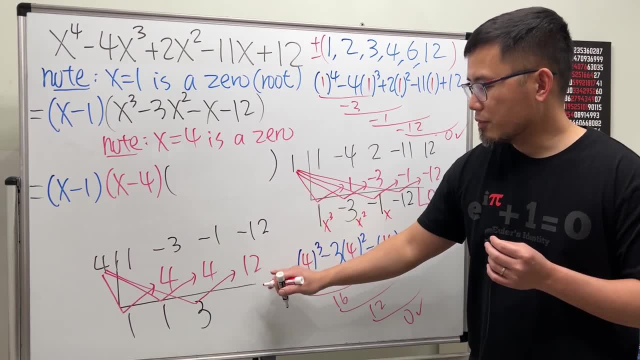 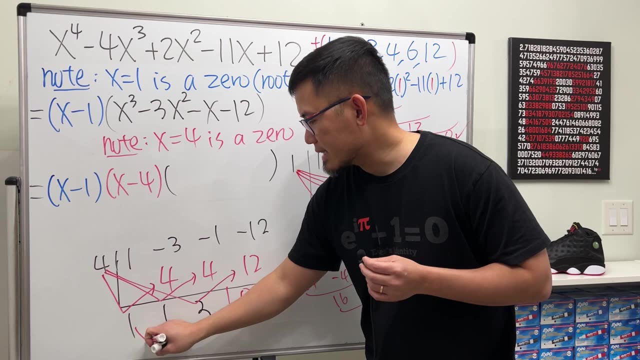 Put it here: Negative 12 plus 12. We end up with 0. So all good. So that means this factor is 1x squared, Because the power goes down by 1. So 1x squared. 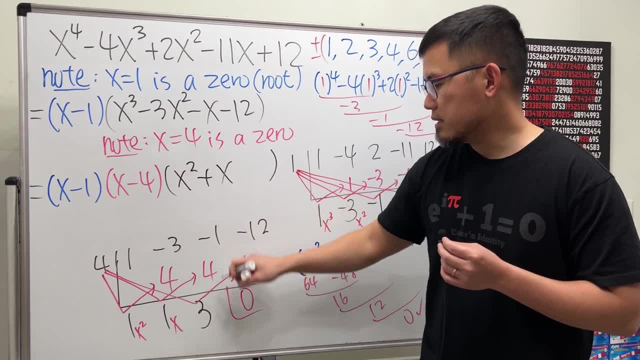 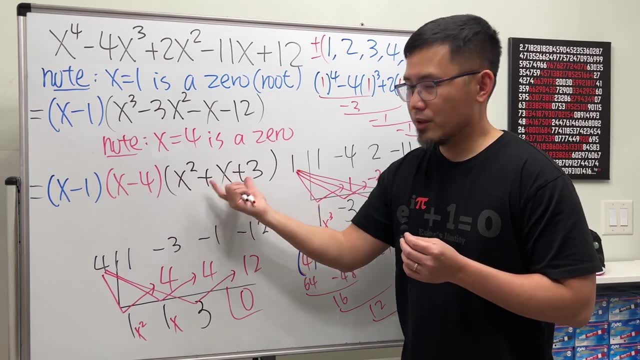 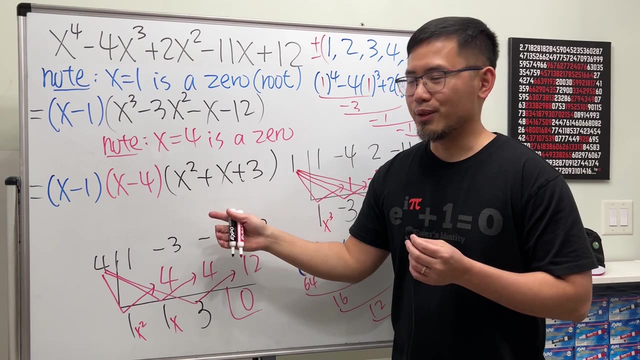 And the next one is positive x And the last one is 3.. Just like that. Now, finally, this is just x, squared Like a regular quadratic trinomial. Can we factor this with real numbers? No, I don't think so, right. 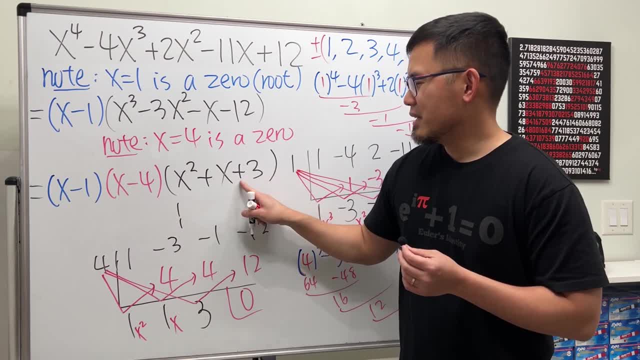 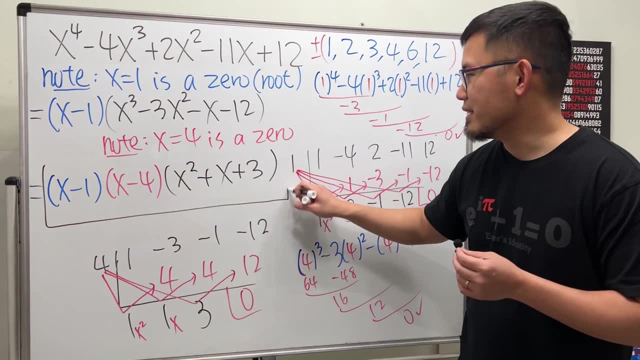 Because this is just 1 and 1.. And this is 3 and 3.. 3 and negative 1.. No matter what you do, this is not factorable. In that case, we know this right here. is it Just like that? 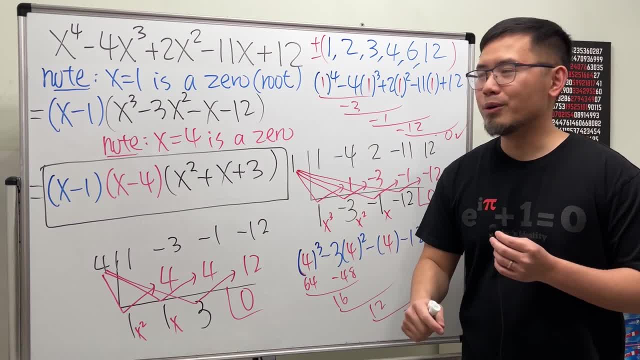 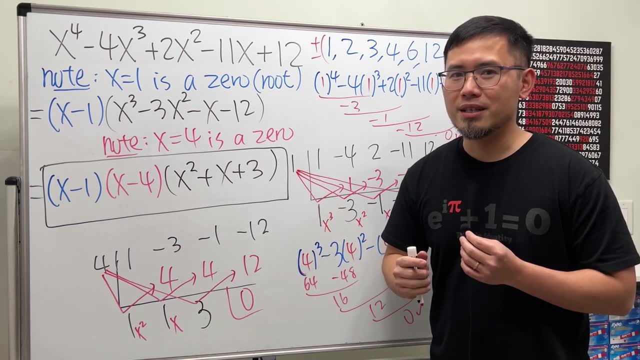 So this is just one way of factoring a 5-term polynomial by using the rational zero theorem and also the sensitivity efficient. Check out my next video because I will show you guys a different method.